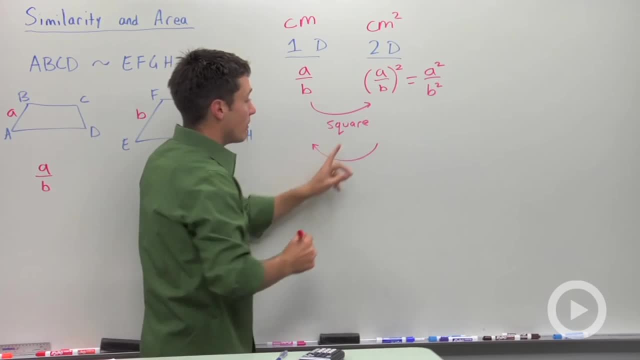 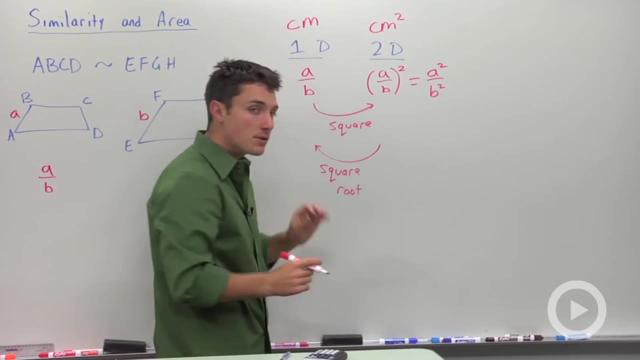 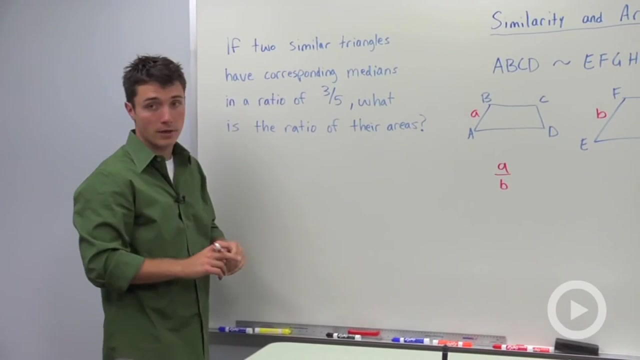 To go in the opposite direction. you're going to have to do the opposite of squaring something which is the square root. Let's look at a brief example of how we can apply this Here. it says: if two similar triangles have corresponding medians. 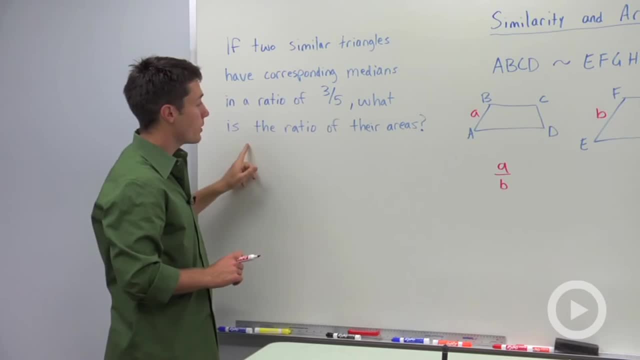 in a ratio of three to five. what is the ratio of their areas? The first thing that will trip up students about this statement is medians. Well, you have to remember that if you have corresponding medians in similar triangles, that they're going to be proportional. 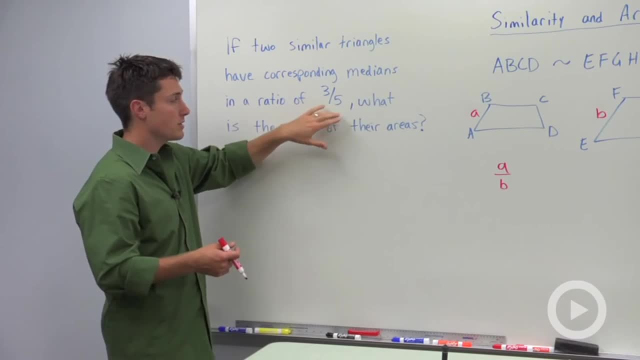 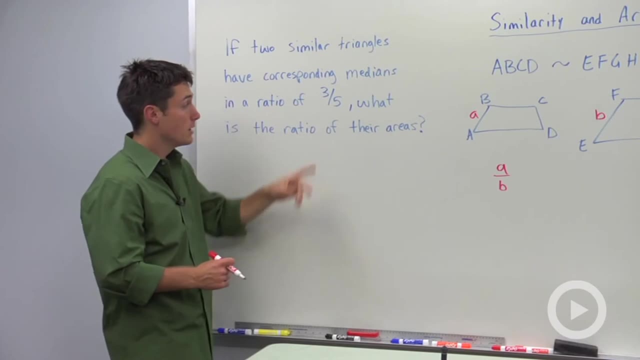 So just because we're talking about medians doesn't change this ratio of three to five. Median is a one-dimensional attribute of this triangle, It's a distance. So this ratio of three to five I can write under the category of one-dimensional. 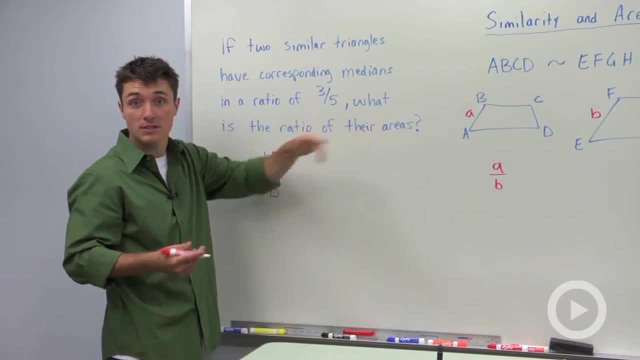 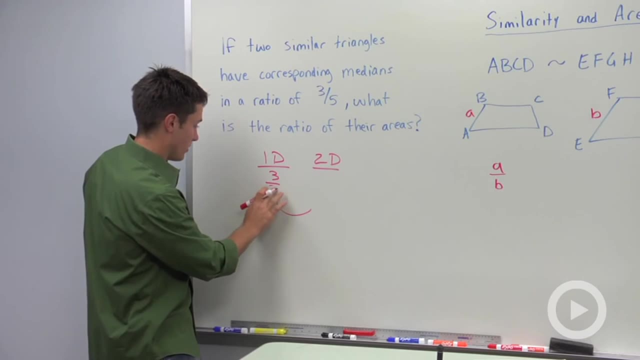 So to go from one dimensions to two dimensions, because it's asking about area, so we want something that's two-dimensional. we know, and actually I don't know what that number is- it's supposed to be three to five. to go from one dimensions to two dimensions, we need to square. 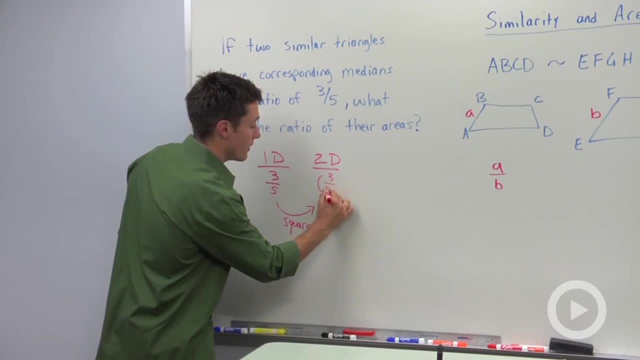 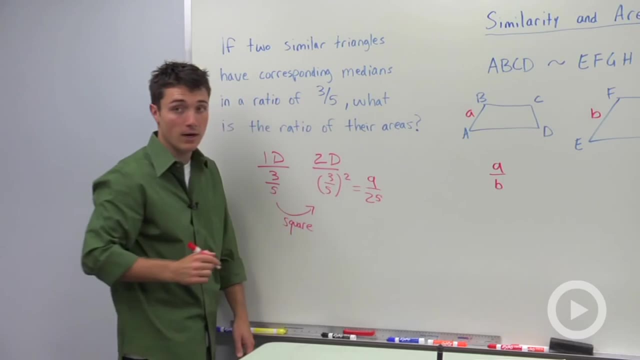 our ratio. So we're going to take three-fifths and square it. So three squared is nine, five squared is twenty-five. So notice that the one-dimensional ratio is three to five and the ratio of their areas will be nine to twenty-five. This is not saying that the ratio is 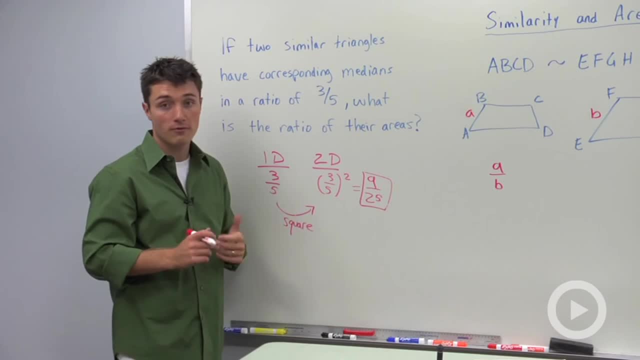 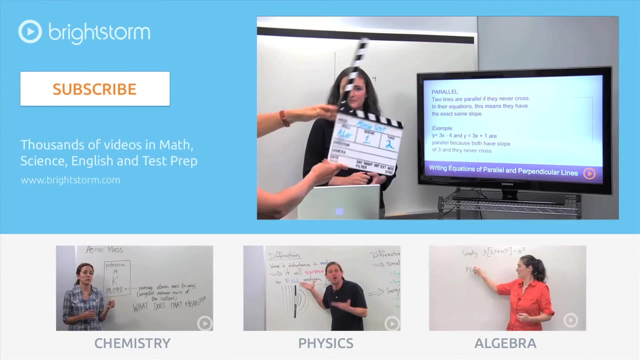 nine, or, excuse me that the area is nine and the area is twenty-five. it's just saying that when you write a ratio of their areas it will be nine to twenty-five. I can't do this with you two laughing back there. 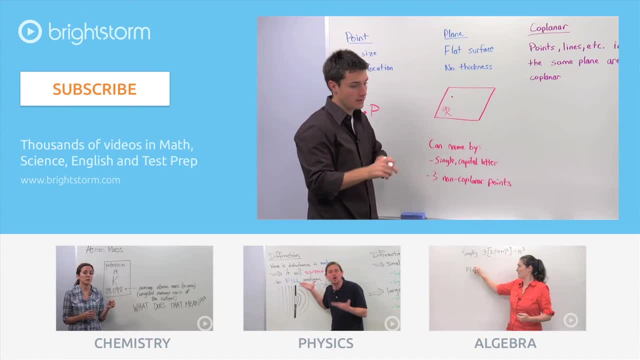 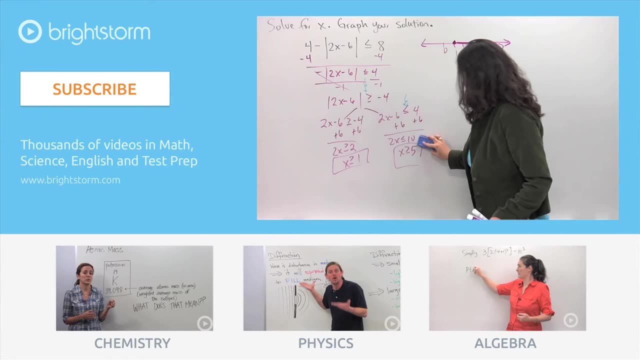 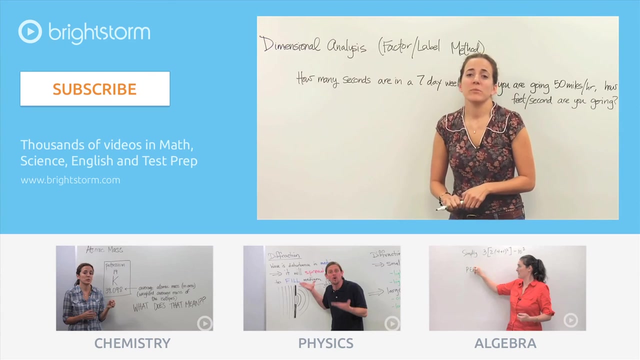 So if we had- no, that's not right- three coplanar points. So have you ever gotten off an airplane? That should be, yeah Dang. Is it like five hundred degrees in here or what? Alright, so when you're in, 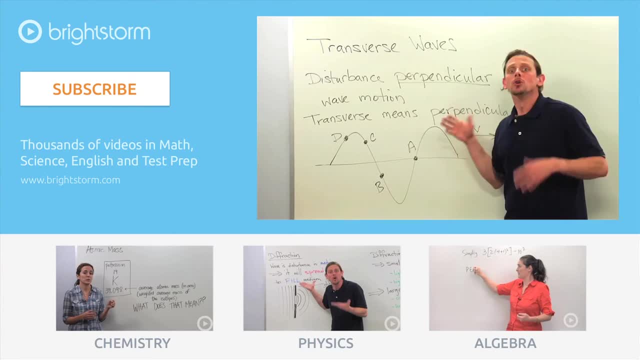 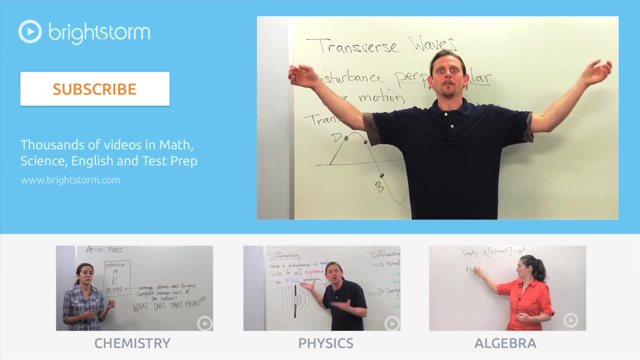 chemistry class. you're going to be doing a lot of work. you're going to be starting over. So, as an example, we could consider: like you've got a chain hanging from two um two-fifths Yeah.